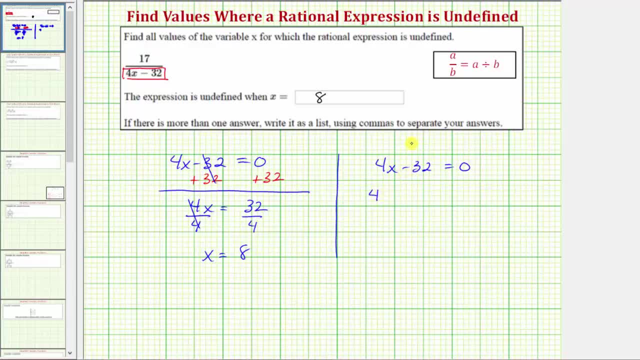 factor is four. The factor four out of the left side would be left with the quantity x minus thirty-two. minus eight, This product is equal to zero. when the factor of x minus eight equals zero, To solve for x we'd add eight to both sides, giving us the same value of x. 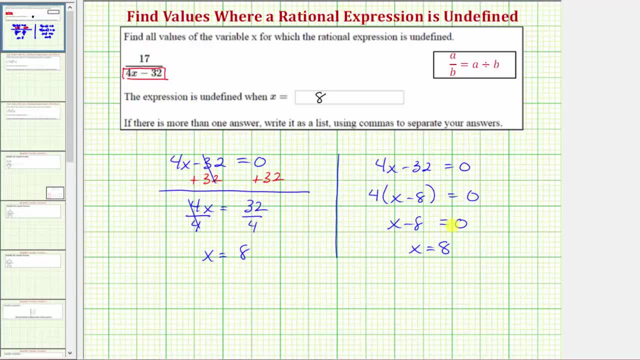 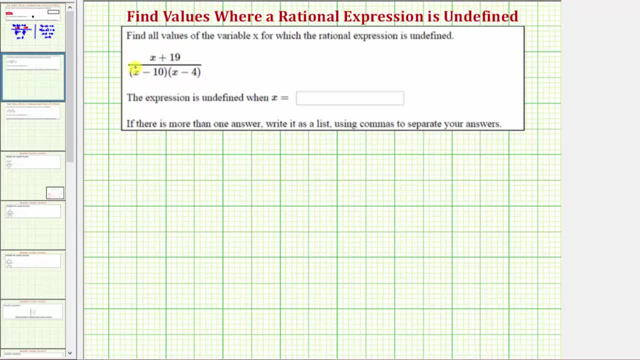 equals eight, where the expression is undefined. In our next example, the only difference here is that we have two binomial factors in the denominator, So this expression is undefined when the quantity x minus 10 times the quantity x minus four is equal to zero. 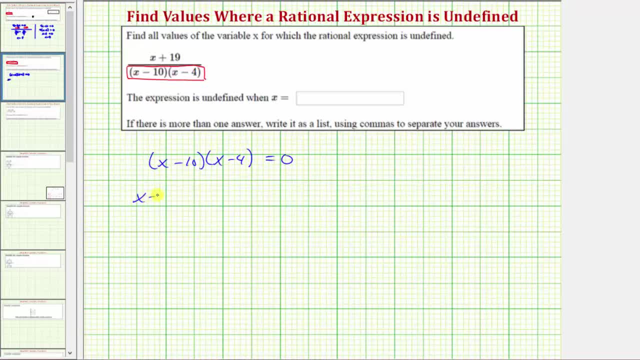 This product equals zero, when the factor of x minus ten equals zero, or when the factor of x minus four is equal to zero. Solving for x: here we add ten to both sides, giving us x equals ten. Solving for x: here we add four to both sides, giving. 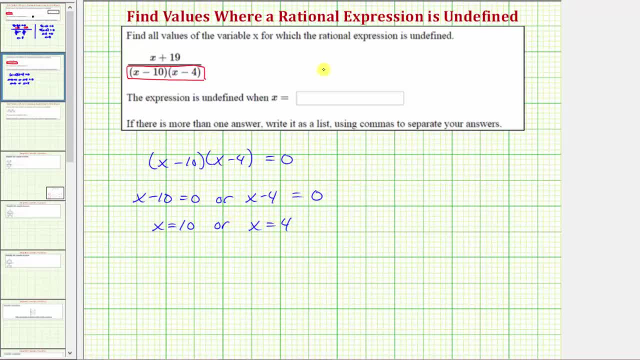 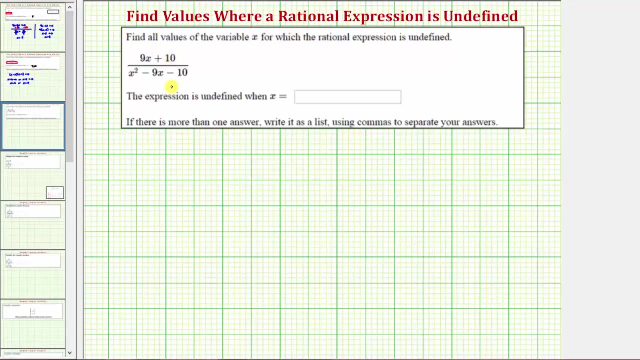 us x equals four, which means the rational expression is undefined when x equals ten. Notice how we do not consider the numerator when determining the values for which a rational expression is undefined. For our last example, the only difference here is the denominator is not in factored form. The rational expression is undefined, meaning we 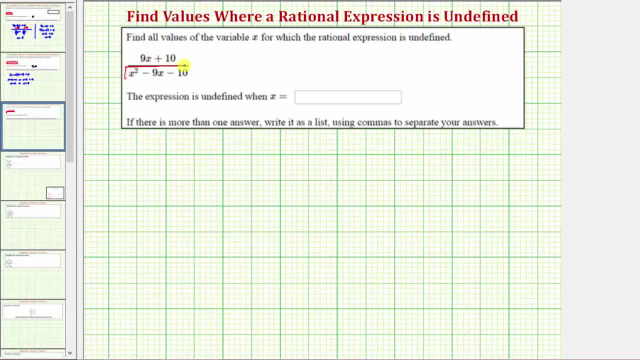 have division by zero when the quantity x squared minus nine, x minus ten is equal to zero. So the left side factors into two binomial factors, Because the first term is x squared. we have a factor of x here and x here in the first positions of the. 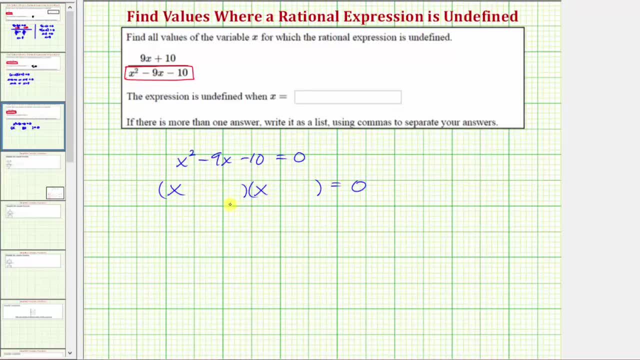 binomial factors. And then for the second terms in the binomial factors, we're looking for the factors of negative ten that add to negative nine, Because negative ten times one equals negative ten and negative ten plus one equals negative nine. the two factors we're looking for are negative ten and positive one, So one factor would be x.